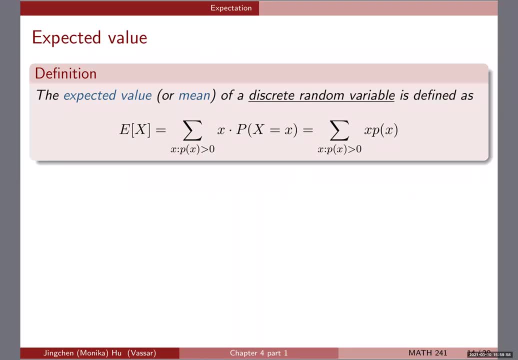 or average of a discrete random variable. So notice that we highlight here this works, for discrete random variable is defined to be so the notation here we use a capital E to represent the expectation Okay, And we typically use a bracket or parenthesis of. 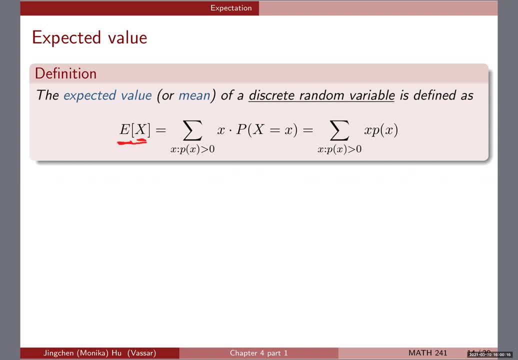 the random variable inside to represent the expected value of random variable X. Okay, So mathematically, what that is doing is that we are multiplying with the possible value, like any value, any possible value of the capital: X. Okay, Multiply that. 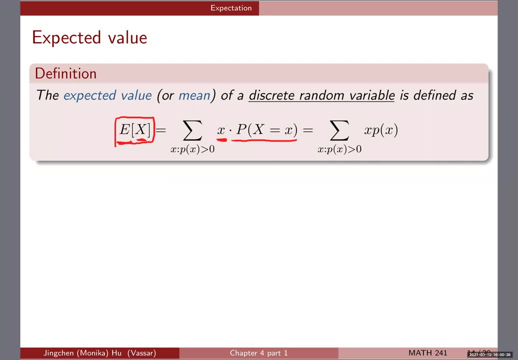 with the PMF evaluated at this value. So PMF- if you remember so eternally, we can also write it over there. We take the product of the two and then we sum that over to all of the possible values that X can take where its PMF is positive. 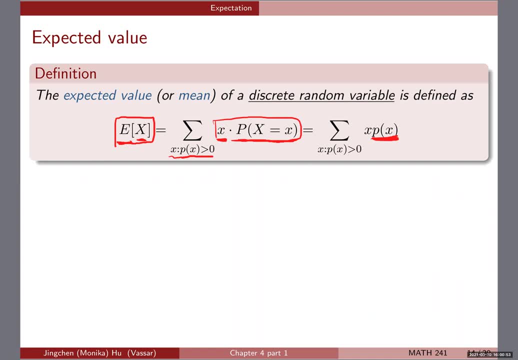 Okay, So it could be that, remember, sometimes we could have a PMF evaluated at a certain point equals to zero, Because if that is the case, then this whole PMF value becomes zero. So that term goes out of the summation. 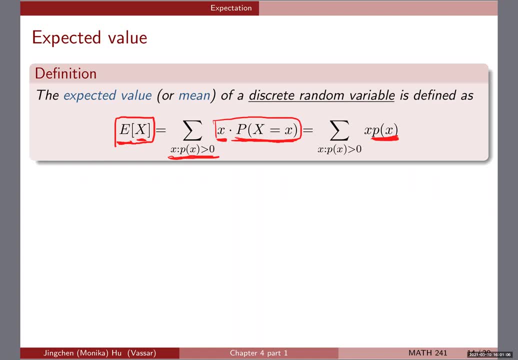 So that's why we really just talking about looking at the possible values of capital X, like among all of the small x over here, that is, having a positive probability, Okay. So equivalently, because this is the PMF right, Evaluate a small x. so we 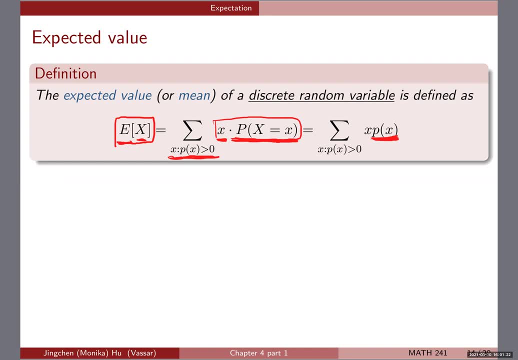 can always write it over there as well. So the way to understand it. okay, It is a weighted average of the possible values, small x, that the capital value, capital X, which is the random variable, can take on, each value being weighted by the probability of Px. okay. 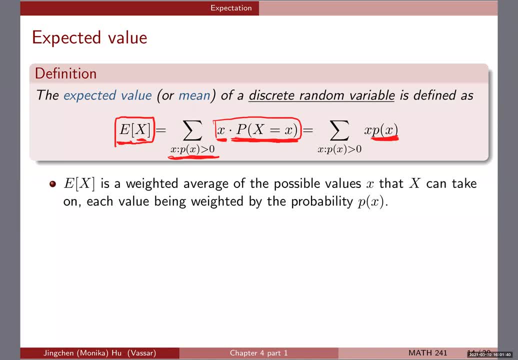 So in English- plain English, that's what we understand. okay, And mathematically we do have the expression for the expected value for discrete random variable. So we can always go back to this definition when we're trying to figure out the expectation for a particular random variable. okay, 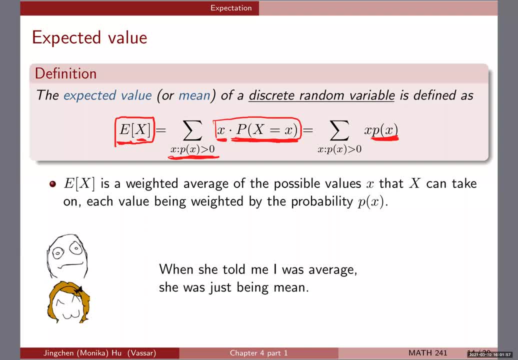 And also, since people are talking about like average, mean and expectation, there is a joke that when she told me I was average, she was just being mean, so I was just hoping to share that with you all. Let me clear that up, okay. 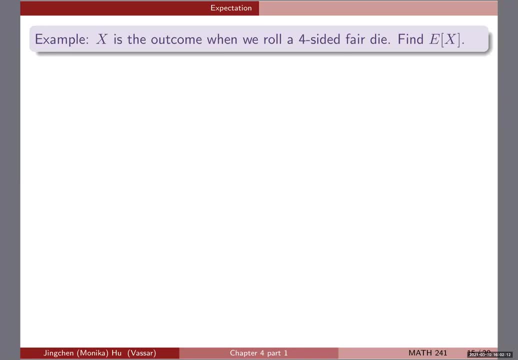 So let's look at example and try to find its expectation. just to make sure that we know how to work it out using the expectation definition. okay, So x is the outcome when we wrote a four-sided fair die. Find the probability, find the expectation of x- okay. 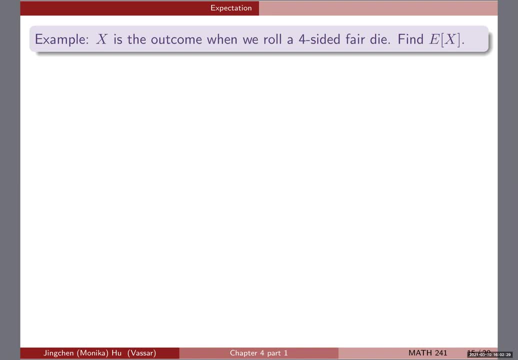 So just to get us started, okay, Expectation of x based on the definition before. okay, It's looking at all of the possible right. The PMF is greater than 0, and we're having x times px. okay. 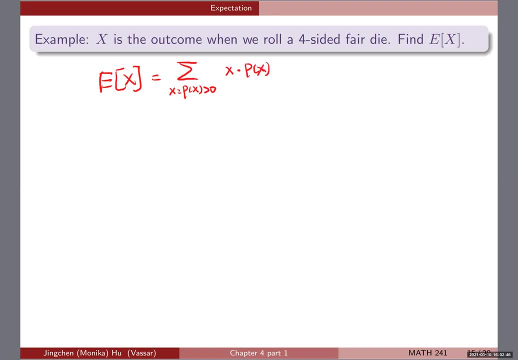 x is the value of. so all of this is small x, okay, Except for this one. this is cap to x, okay, So, and here, small, small as well. So small x. here is the value, each of the possible values. 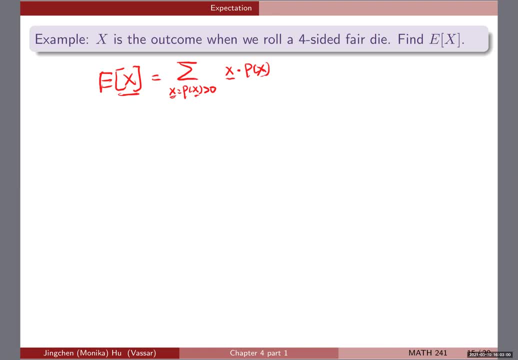 which is one of the four values that can take, right, And then this px, remember, is the PMF. okay, So let's, if you are so familiar and comfortable, you can just proceed this way. But if you're worried about, 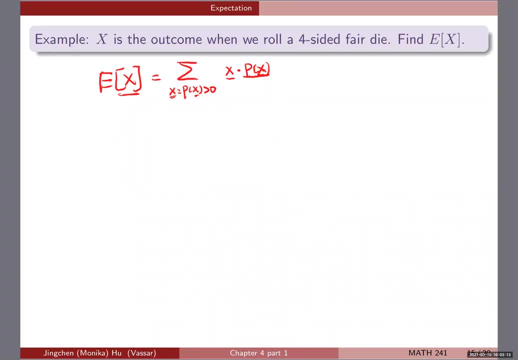 or like just trying to want to make sure that you get every piece correct. maybe one thing we could do just outside of the equation over here is just to show that well, the PMF evaluated at all of the four possible values. 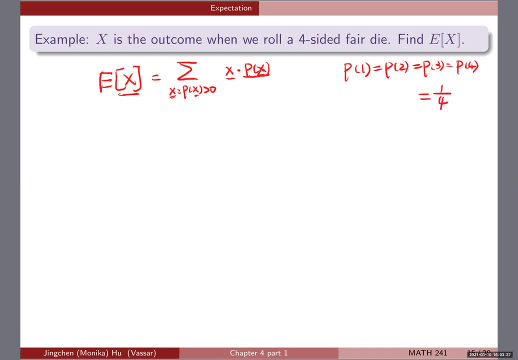 they're the same as one over four, because it's a fair die, Okay. So if I follow this, okay, what this gives me is that: okay, I'm looking at all of the possible PMF values, right, So it's going to be one, two, three, four over here. 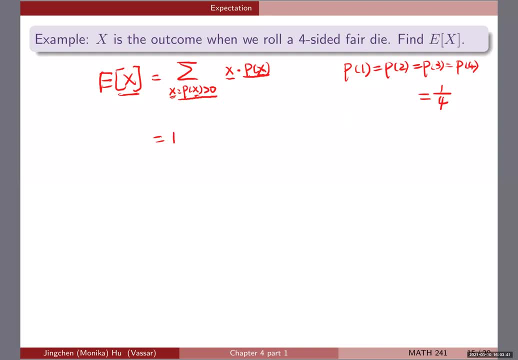 So, if I follow this directly, what this does is I'm doing one times right, One over four, because my first possible value is one and the p1 is one over four. I do that with two, I do that with three. 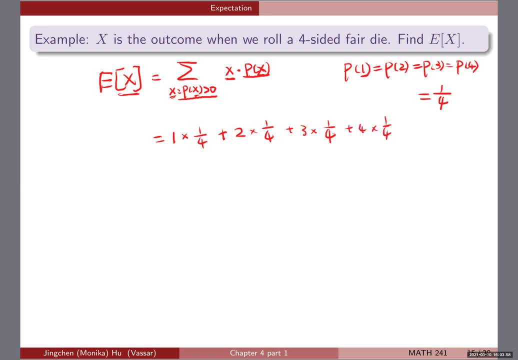 and then I do that with four, okay. If I do it, it's going to be 2.5 or 10 over four, okay. So what this is saying is that if I'm looking at the outcome of rolling a four sided fair die on expectation,